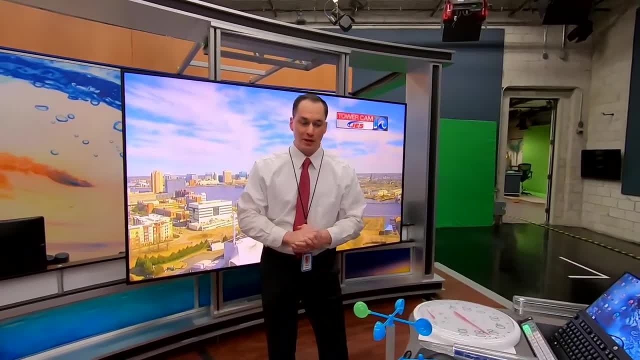 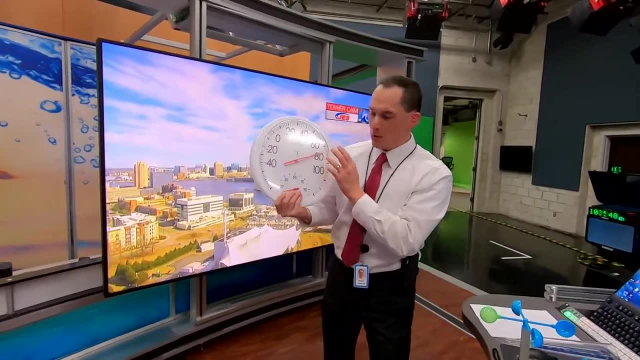 All right, these are some of the tools that we use to understand the weather, and many of them are for observation, Some of them are for prediction. We'll take a look at that, And so here we go. This is the first tool that I use. It's the most important but most simple tool. It's a thermometer. 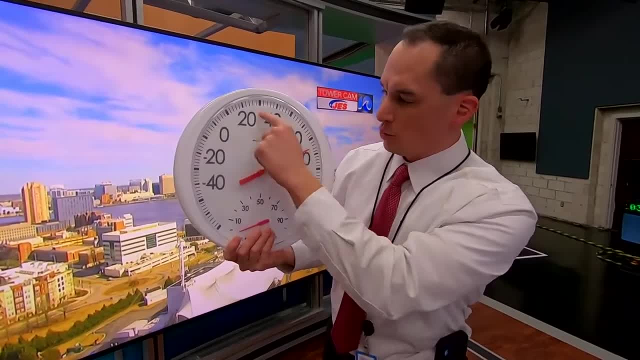 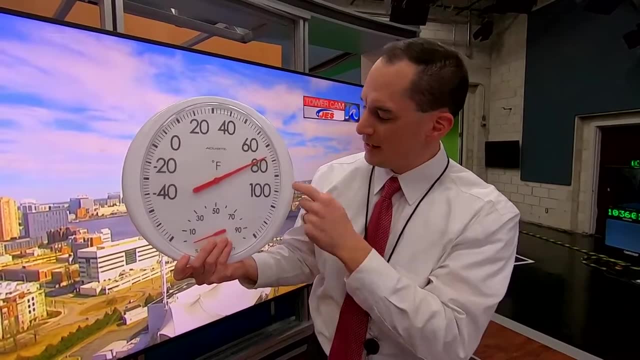 and it measures the temperature. The hotter it is, the more over to this side it goes. The colder it is, the more over to this side it goes. I've been in temperatures down to about minus 18 before- I'm from Illinois, so that's how that happened- And then I've been up to temperatures about 106. 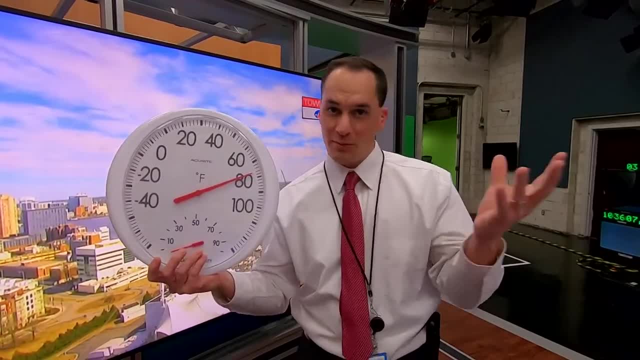 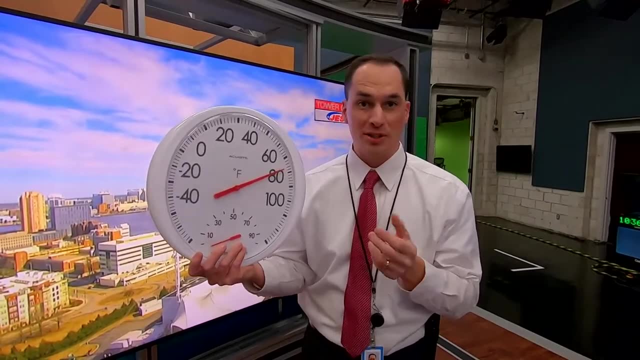 And then so the hotter it is, of course, we tell people: hey, you know, you may have to wear shorts today, or maybe it's super cold outside, You need to wear gear, And so this tool allows me to help you to know what to expect when you go outside. This is the next tool that we have. This is the 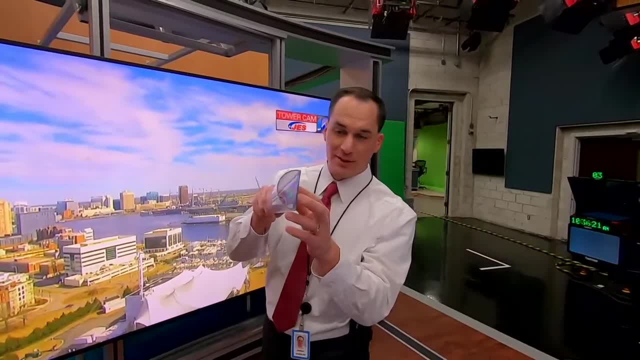 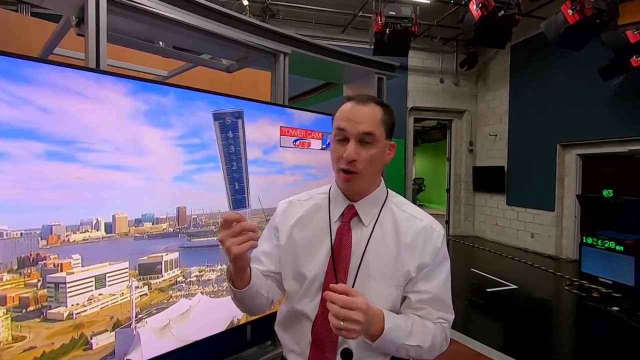 rain gauge. Rain gauge is very simple. The raindrops plop on the top. That's it. It's calibrated And so maybe it rains two inches. you dump it out, you get another rain the next day, an inch- and then you add it up. Weather watches do that for me. That's also a very important job. 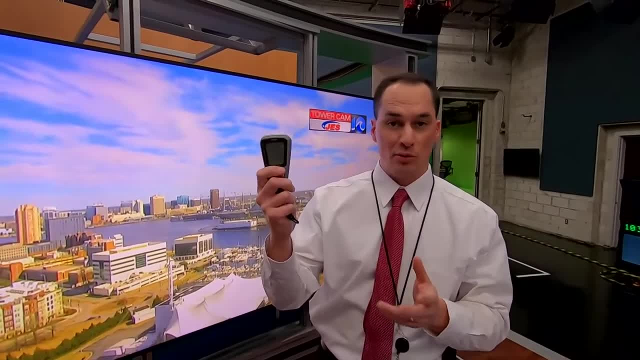 This one not on right now, but I'm going to show you how to do it. I'm going to show you how to do it. This one not on right now, but a very important, as it is the barometer. Barometer measures pressure. Pressure goes up. 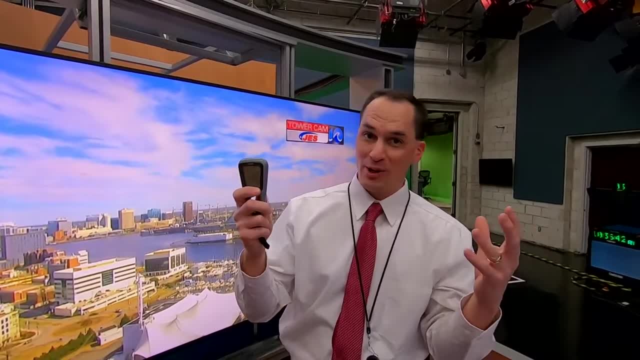 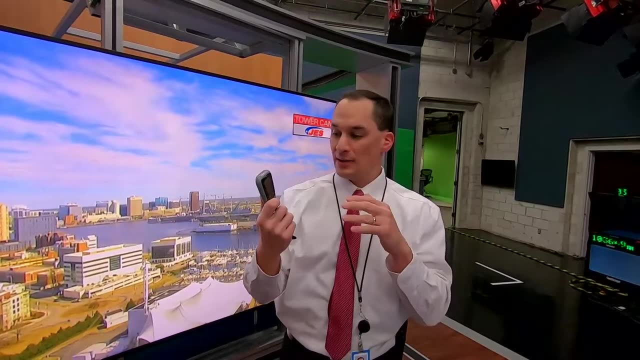 the number goes up, pressure goes down. this drops. When you have high pressure you get happy weather and sunshine, And then when it goes down, you get bad weather. rain, showers, thunderstorms and then tornadoes and hurricanes are extreme areas of low pressure. So this will 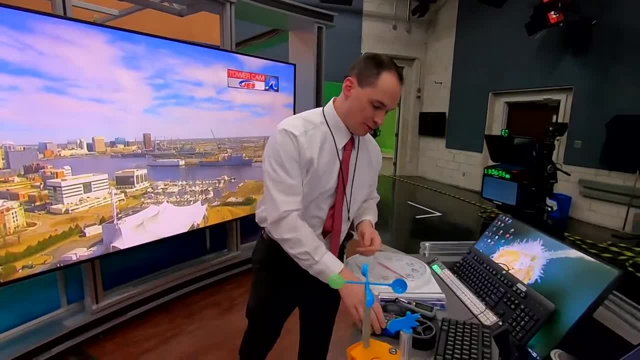 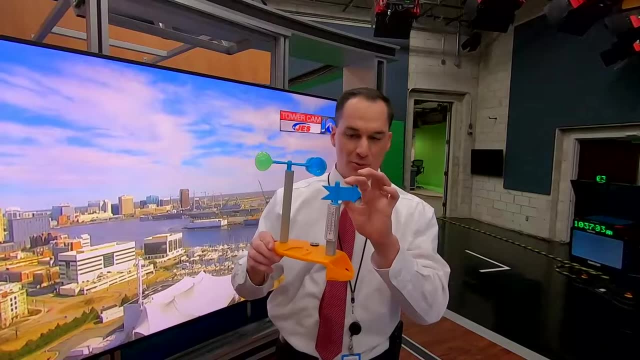 drop and you'll know the storm system's coming. Now, when the storms do come, then we use these instruments to try and figure out the wind. This one is the weather vane just moves in the direction the wind's blowing. It's that simple. This one's a little more complicated, though This: 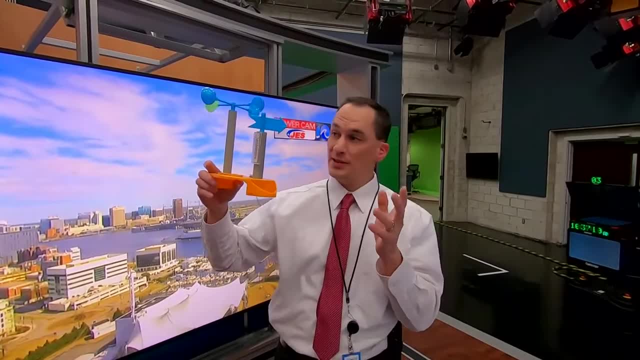 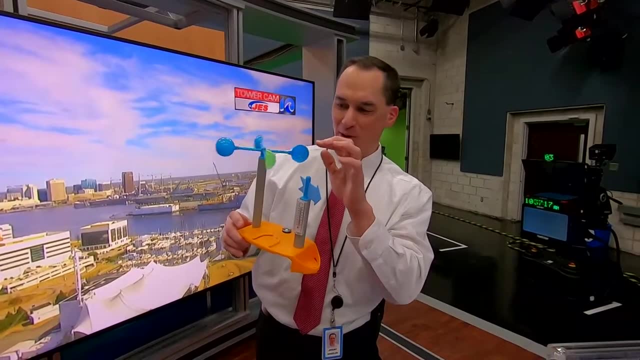 is the anemometer that measures the wind speed. Storm chasers put these on top of their vehicles and drive out to the storms and measure the winds, And so you can actually measure it by counting the number of times the green cup goes around in a circle. measure by a number in a. 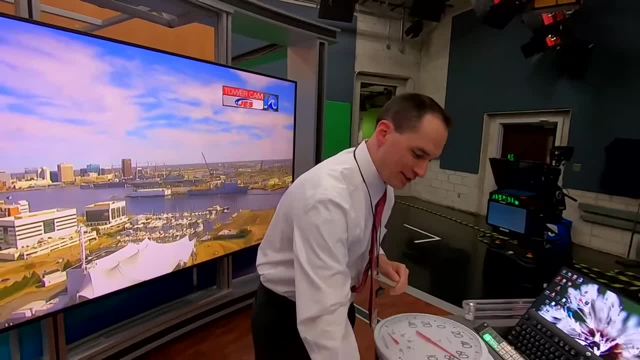 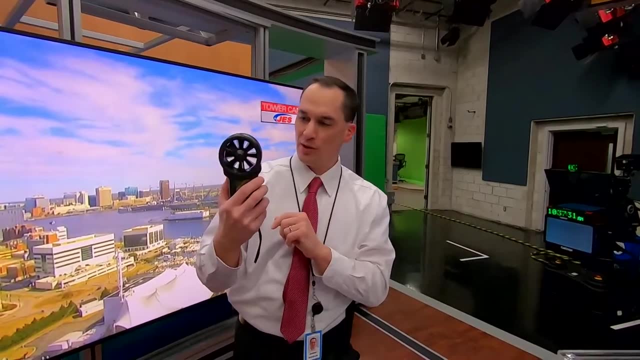 minute and you'll get the wind speed. Of course, we have ones that are electronic that do that for you, And I highly recommend it because when the wind's really going it's tough to count that. So this is my electronic anemometer And this one measures it. especially when you're in a storm It's very. 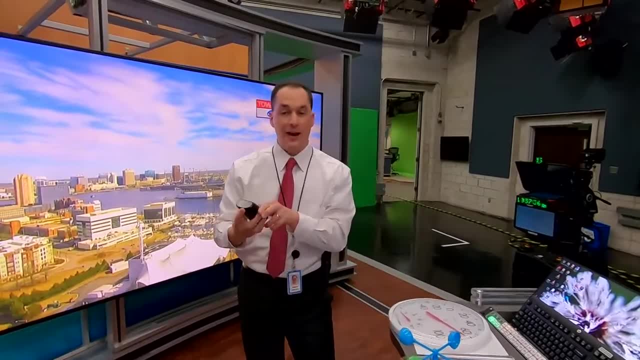 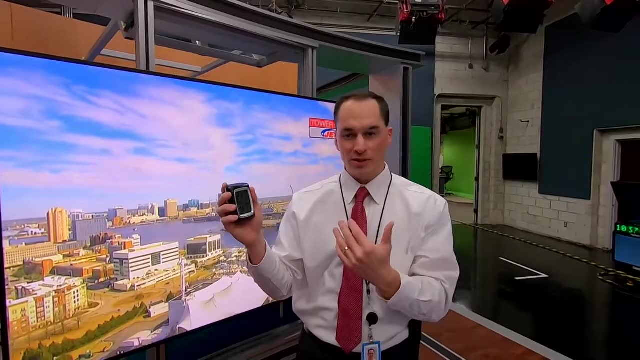 handy to have. This is another instrument. This is called a hygrometer. It measures the humidity and the temperature, And so right now it's 21%. It's very dry inside. When it's in the wintertime, usually you do get a lot of dry air inside, And then, when it's summertime, outside your air 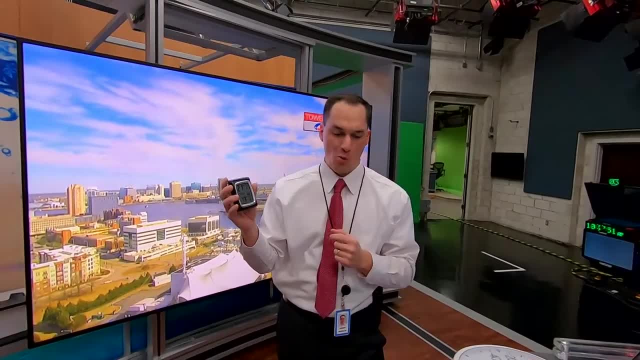 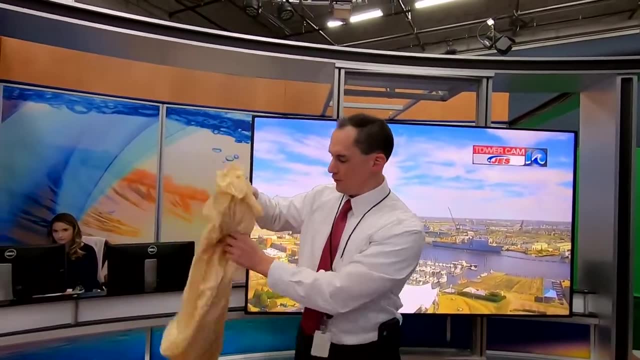 conditioner is running. usually it's the opposite: It might be a little humid inside your home. Now, this is one last tool that we have. We don't exactly use this one. This is on loan from the National Weather Service. This is a weather balloon, and it's a giant weather balloon. 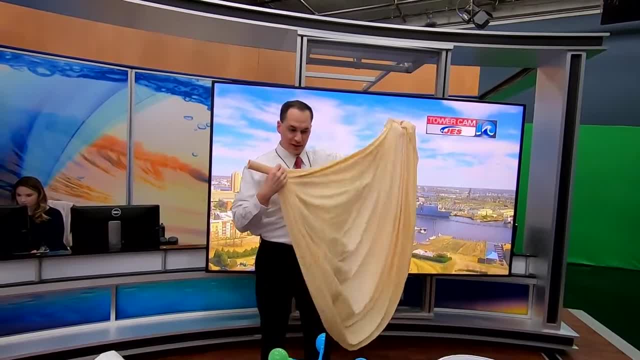 And so they sent this to us. This is a giant weather balloon, and it's a giant weather balloon, And so they sent these up twice a day to measure all of these things, or many of these things, up high in the sky, Because we can measure what's going on at the surface, but you also have to measure what's going. 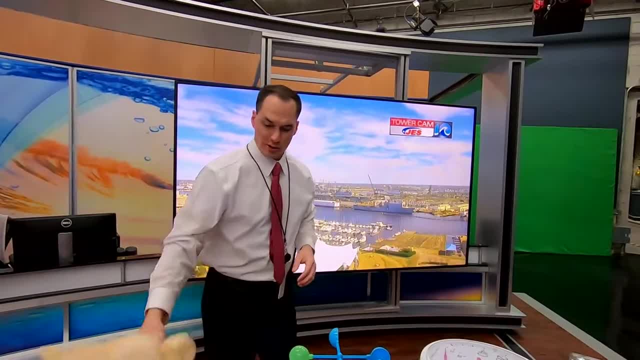 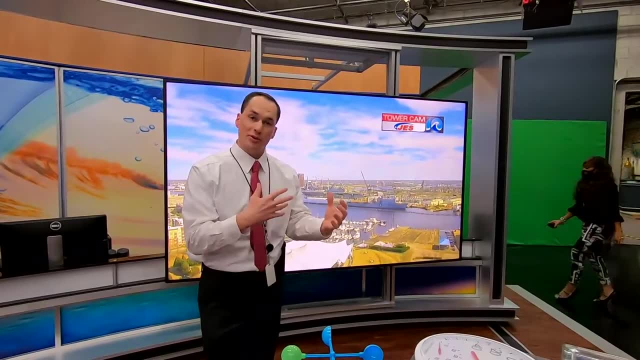 on up here to really get a good idea of the atmosphere, And so those are some of the tools that I use that are physical. Now. I usually don't handle these myself. They're electronic instruments, usually now, and so they'll send me the information. And so we do have some other instruments that are 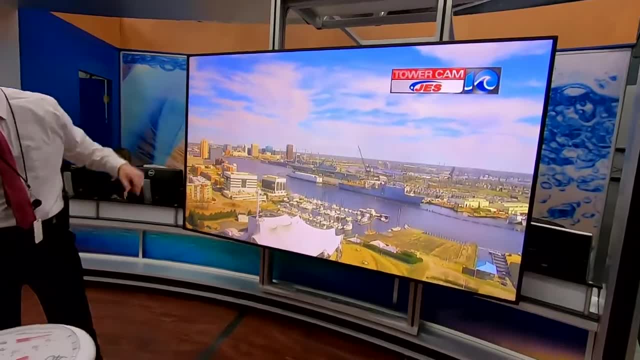 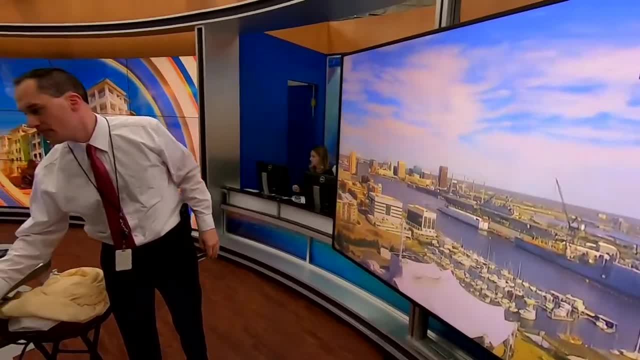 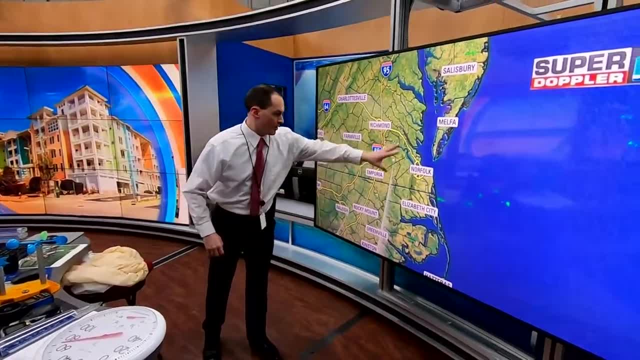 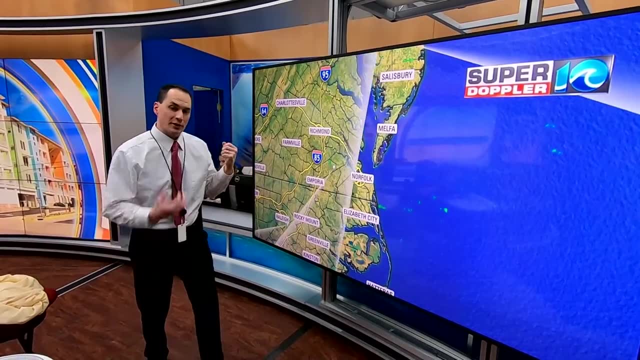 tool. This one is called a radar And this one- there's radars all over the country We use. the information shoots a beam of energy out over the sky. That energy bounces off of liquid water in the atmosphere. comes back, tells us information about where the rain's located, how heavy it is. 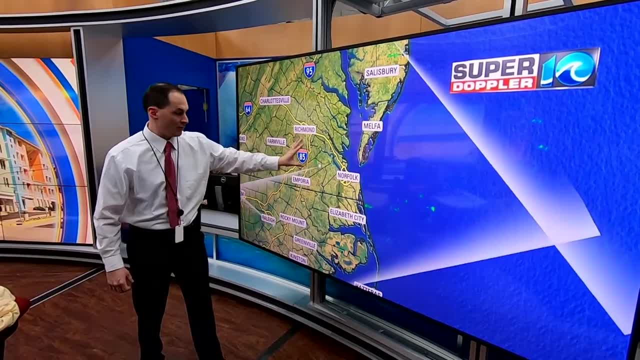 where it's moving to and how fast it's moving, And we use this to track storms and we also use it to track tornadoes. So that's very important. Now, this is another tool that we use: satellites. satellites- Now, this is another tool that we use. satellites: Now, this is another tool that we use. 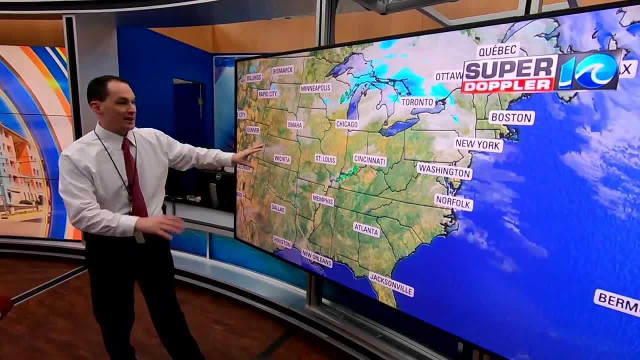 satellites. Now, this is another tool that we use: satellites. Satellites are in space. They look down at the earth. they can tell us where the clouds are and we can expand it. We can look across the entire planet and look for possible storms or even hurricanes. We can track weather.